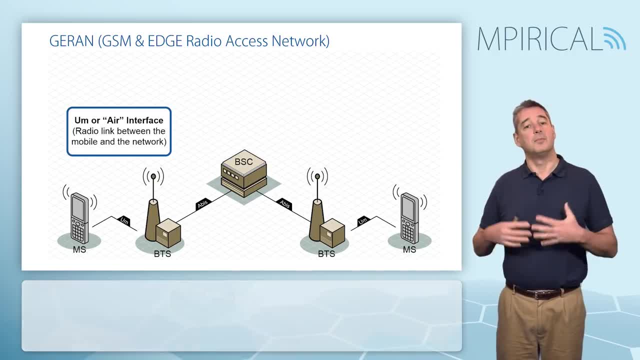 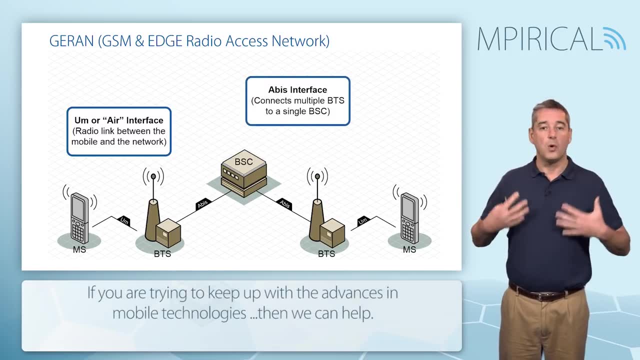 From the base stations or the base transceiver stations, we connect to the base station controller- another key element of our GRAN- via the ABIS interface. Now, it's important to stress these interfaces, for it is these and the messages that pass across them. 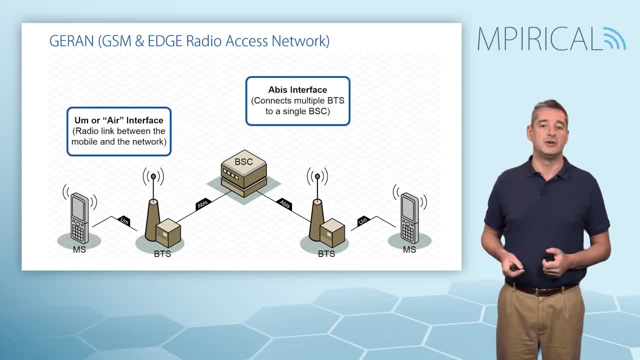 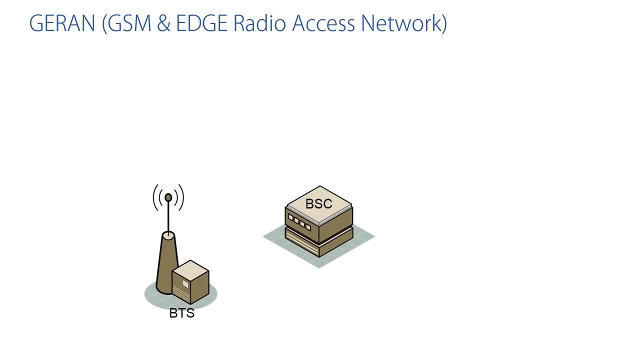 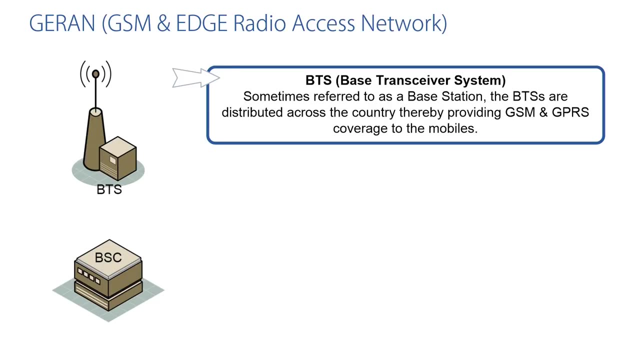 which are defined by the 3GPP, the Third Generation Partnership Project. So let's take a look, then, at the two key elements which comprise of the GRAN. Here we have the BTS, or the Base Transceiver Station, And the Base Transceiver Stations, or Base Stations in the more commonly known. 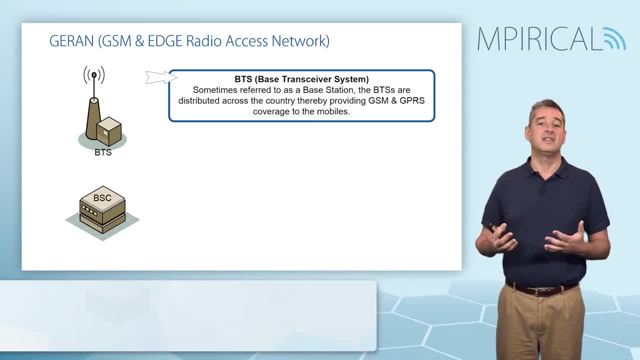 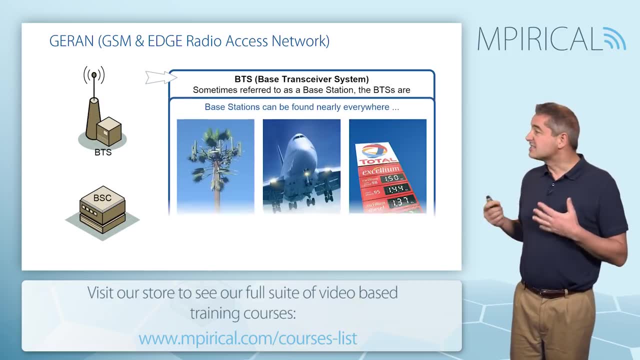 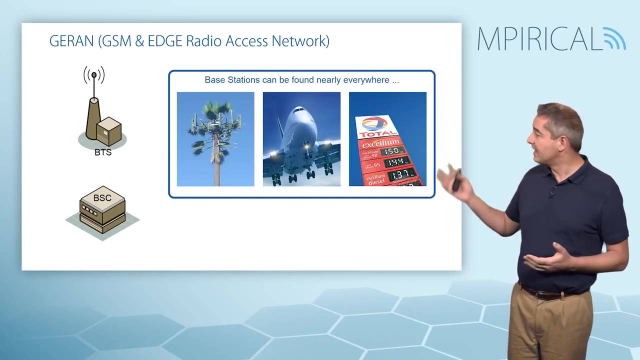 provide us with our coverage across the network. We see these distributed around the countryside, by the sides of roads, on the tops of buildings, etc. It's not uncommon now to find these base stations hidden in other pieces of architecture, possibly disguised as trees, hidden in street furniture or, nowadays, embedded within transportation systems. 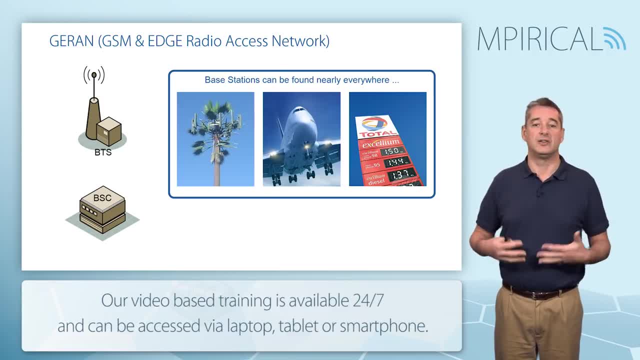 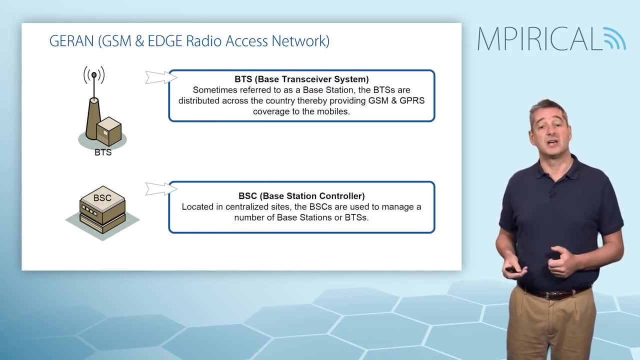 Here we can see on an aeroplane, but also on trains, Ships, trains, coaches, etc. etc. The second element, then, of our GRAN is the Base Station Controller, And, as the name would suggest, the Base Station Controller controls base stations. 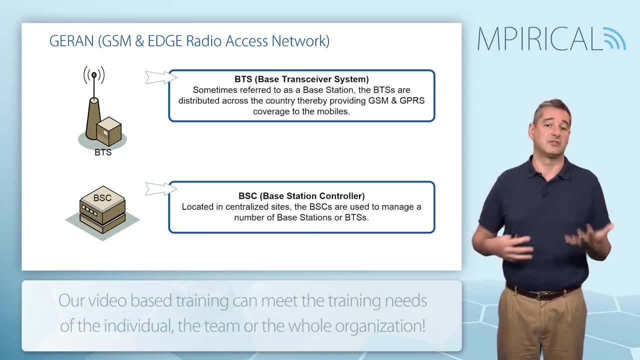 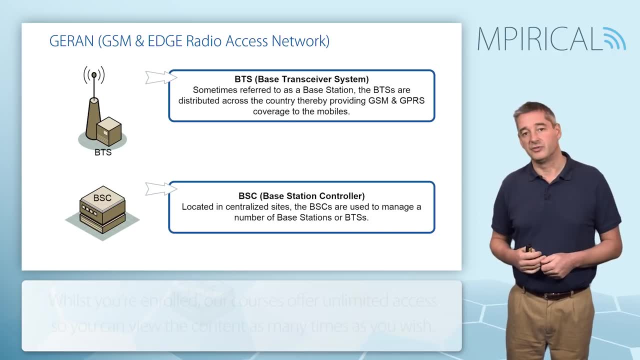 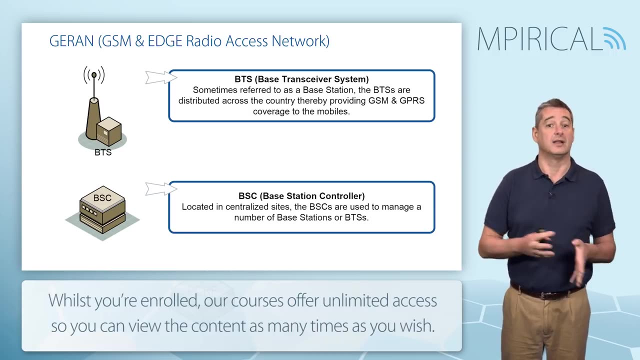 But it will also control the mobile as well, in terms of things like power control, telling the mobile to increase or decrease its power as it moves further away from the base stations. The Base Station Controller will also deal with handovers as well, so it's a very important decision to move the phone from one cell to another. 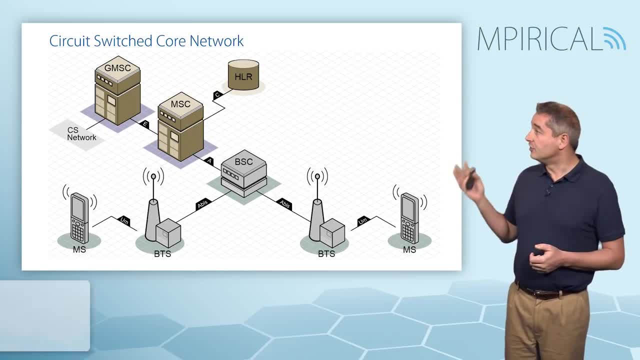 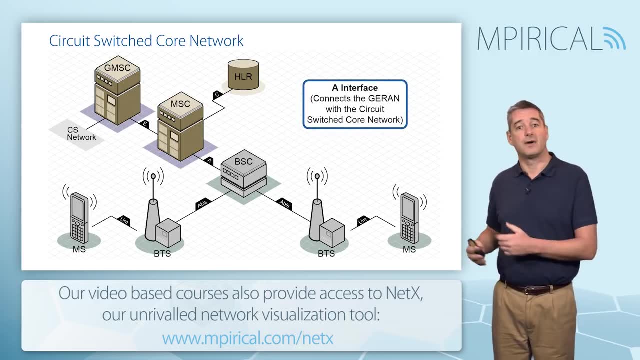 Now, as we leave our GRAN, we can connect up to the core network And to begin with we're going to deal with the circuit switch core. Here we can see it connects back to the GRAN via one of these defined interfaces. 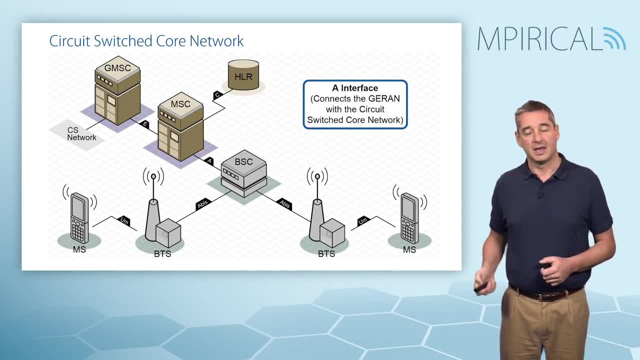 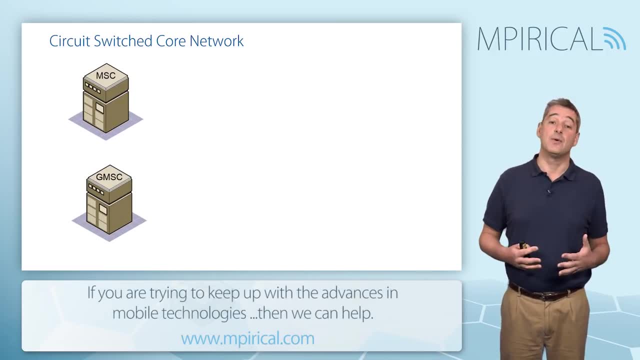 This time we refer to it as the A interface. Now, the circuit switch core is made up of two key elements: The MSC, or Mobile Switching Centre, and the Gateway- MSC, or Gateway Interface. These are the two components that make up the Mobile Switching Centre. 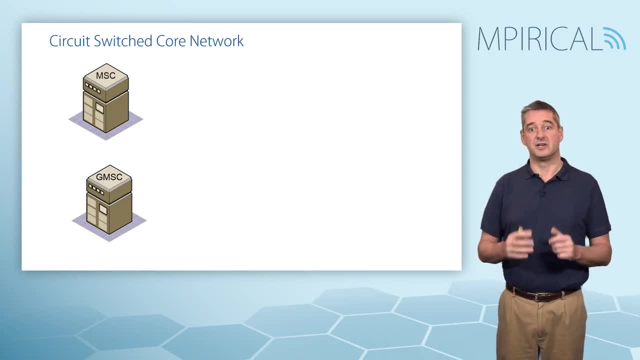 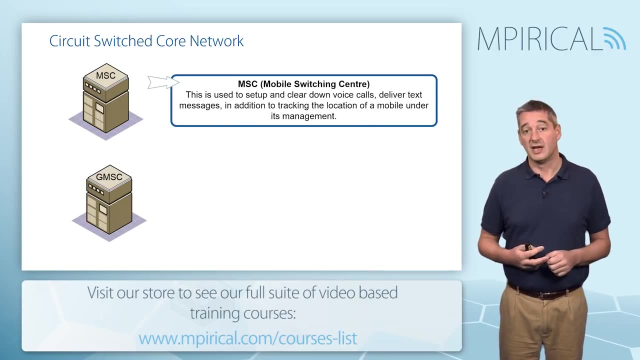 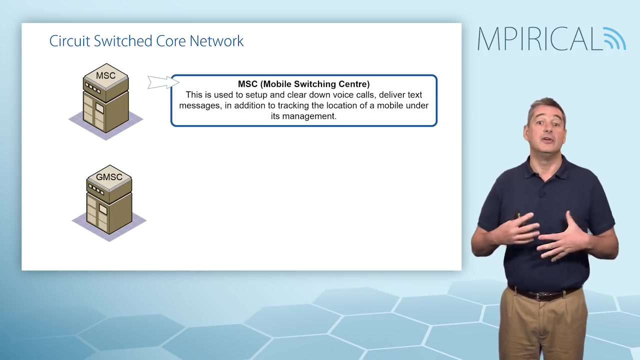 However, it's not uncommon to see both of these functions combined within the same piece of physical architecture. Now, the MSC is responsible for setting up and clearing down telephone calls, sending text messages, etc. But it will also deal with mobility management, tracking the mobile as it moves around the network. 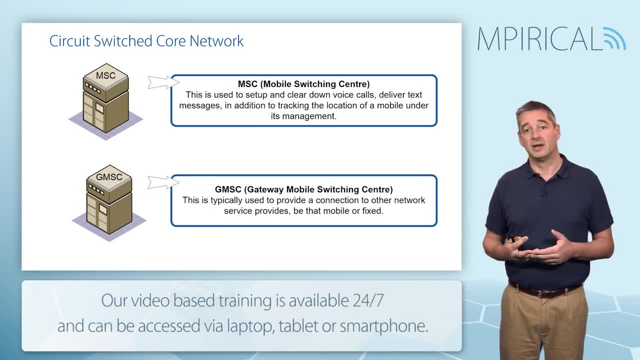 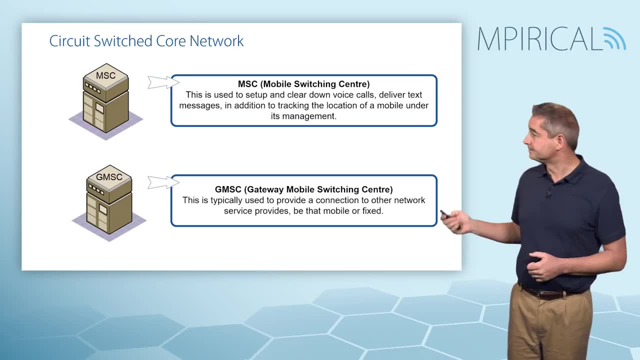 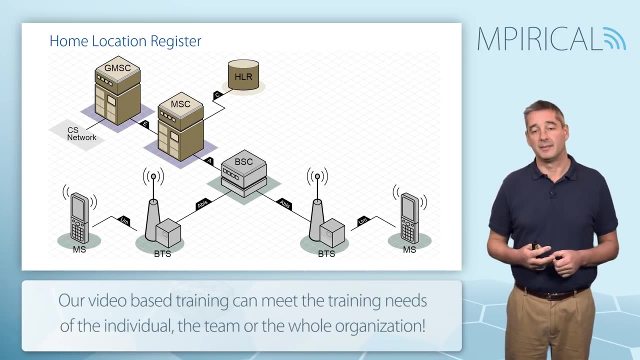 The Gateway MSC provides our form of ingress and egress out of the network. It can control other mobiles or telephones on either mobile or fixed networks. Now, sitting at the top of the screen, we can see we have a database termed the Home Location Register. 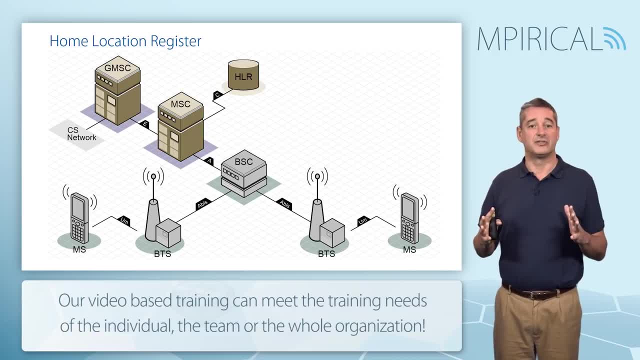 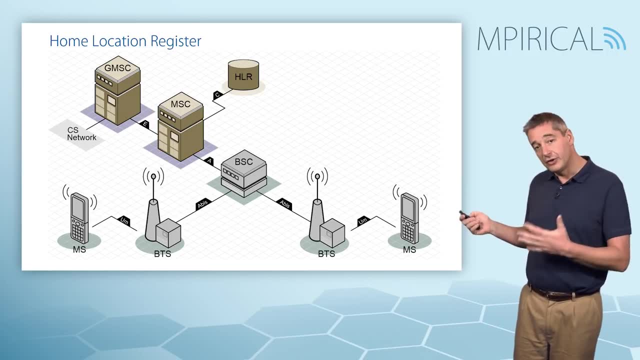 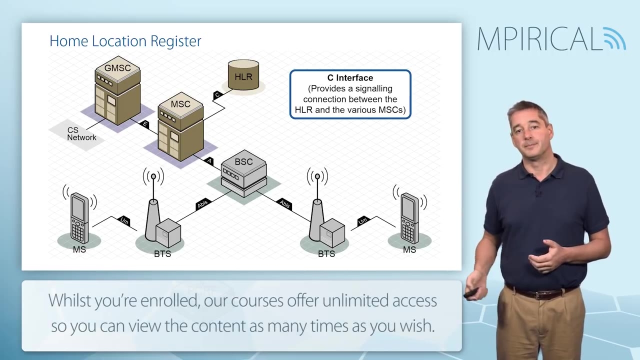 Now the Home Location Register is one master database which contains all the information about the subscribers who belong to this network. It connects to the MSC here via the C interface, which carries signaling information between the two nodes. Now, in reality, a network will not be comprised of a single MSC. 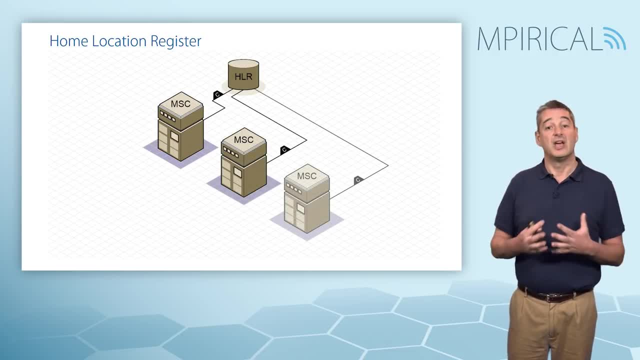 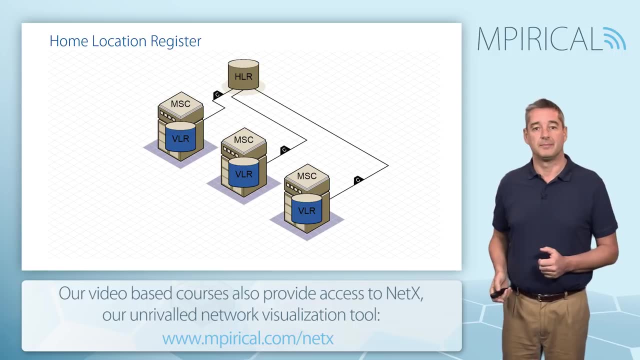 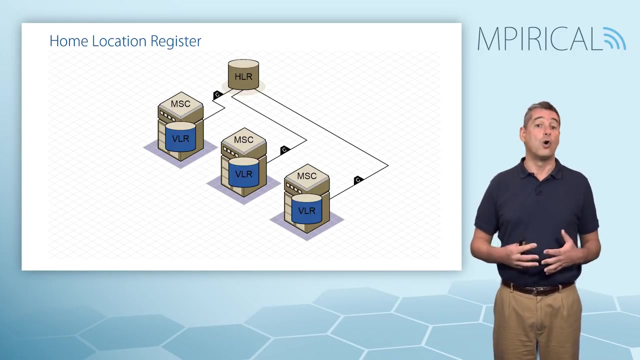 Realistically, there will be a number of MSCs distributed across the network, each one providing historically a region of geographical management. Inside each of these MSCs, there will be a database, and this database is termed the VLR or the Visitor Location Register. 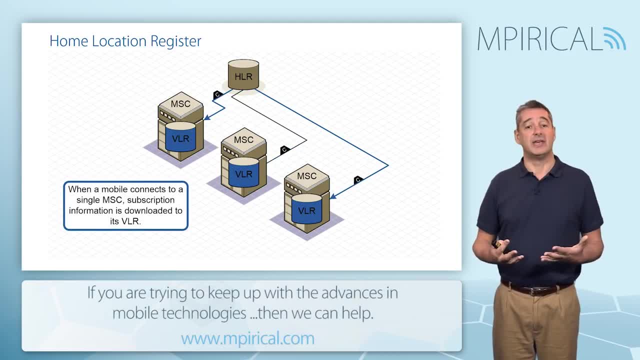 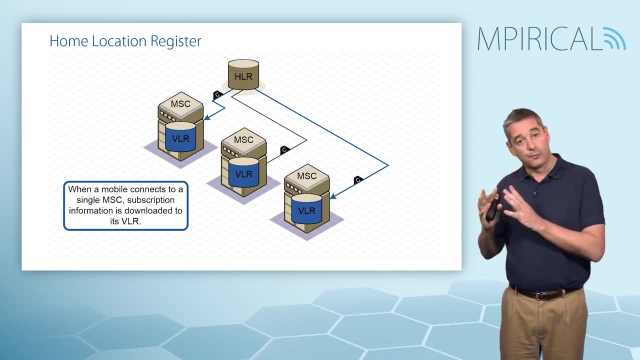 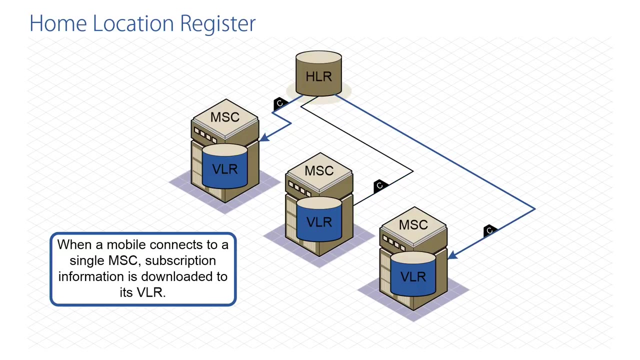 So as a mobile connects up to an MSC, as it attaches to this MSC, then we will download subscription information about this subscriber from the Home Location Register down to the particular MSC VLR that the mobile is operating under And in this way we can carry out local management. 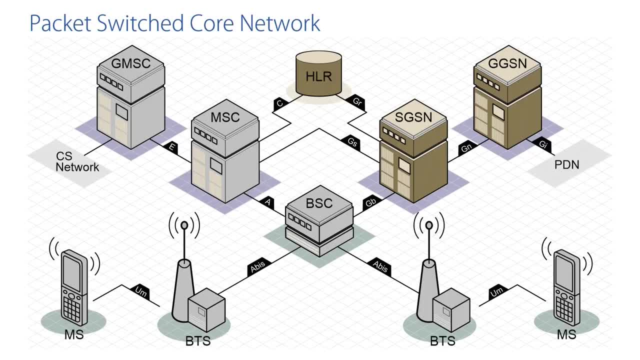 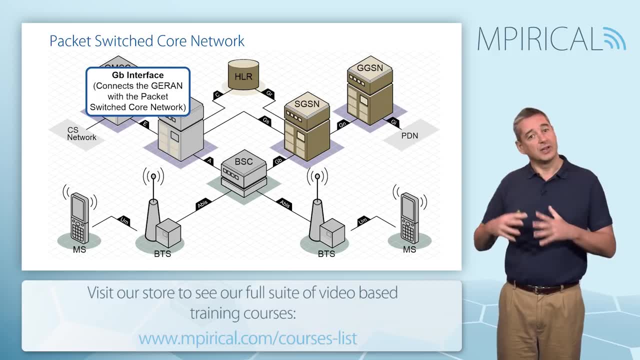 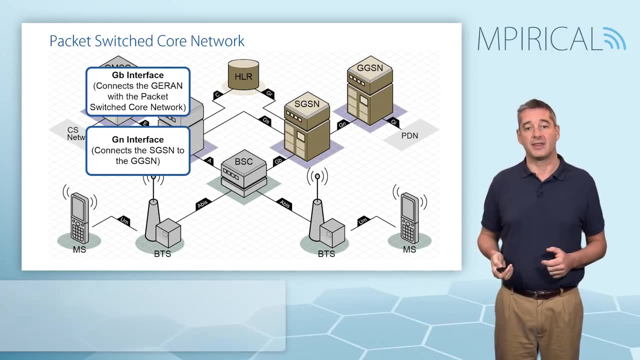 The second element, then, of our core network is the packet switch core network, and it connects once again via various interfaces: The GB interface, which links our packet switch core network to the GRAN, a GN interface which links the various GPRS support nodes together. 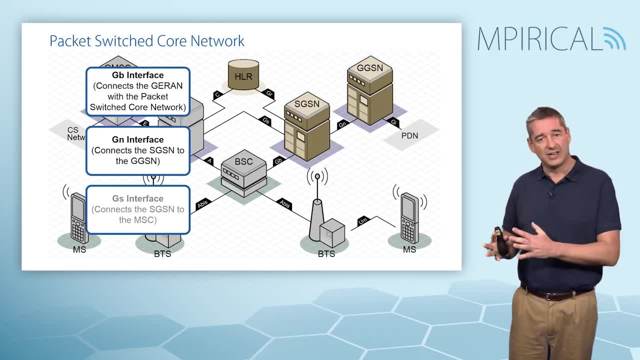 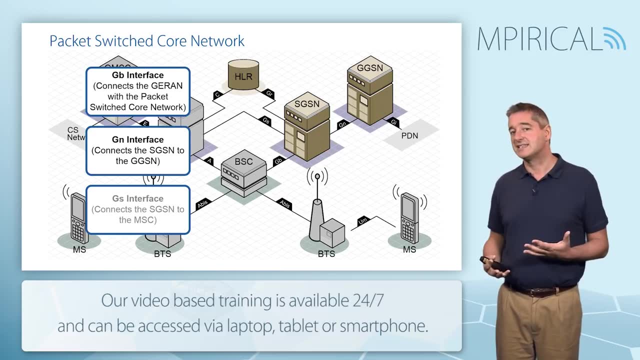 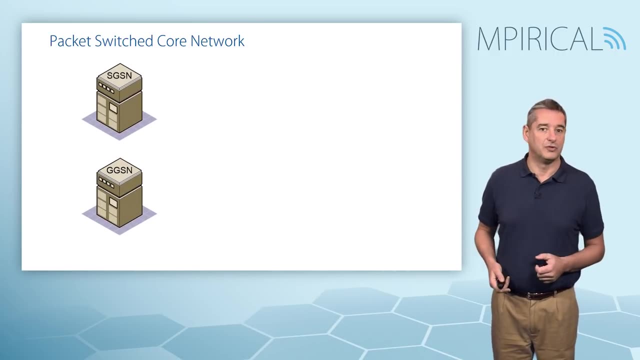 and possibly a GS interface which links our packet switch core to the circuit switch core, Although it must be said that in most networks around the world today the GS interface is seldom found. So looking at the two key network elements in a little bit more detail, 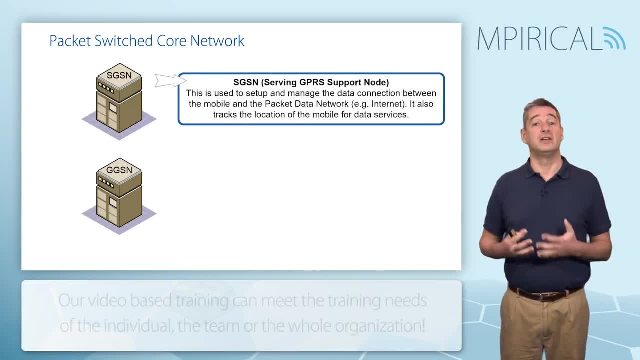 Well, we have the SGSN, or the Serving GPRS Support Node, And this is responsible for the setting up and management of our data connection, the always-on connection we take for granted with GPRS. It, too, deals with mobility management. 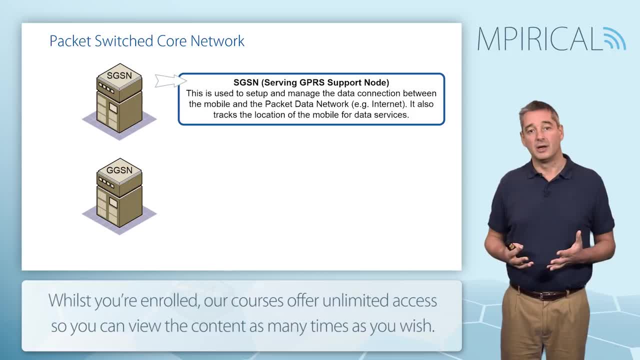 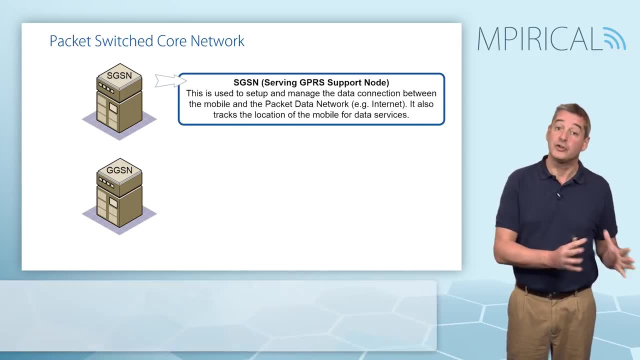 It will track the mobile as it moves around the network, but this time tracking the mobile for packet switch services, whereas my MSC VLR tracks the mobile for circuit switch services. The final element is the GGSN, the Gateway GPRS Support Node.